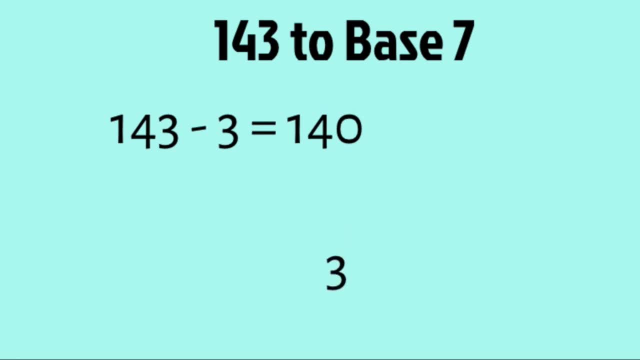 We then add this remainder to the very end of our final answer, With our number 140,. we then divide by the base, which is 7, to get 20.. With this number, we then repeat the process. So we subtract by 6 to get 14,, we add the 6 to the end of our number and then we divide by 7 to get 2,. 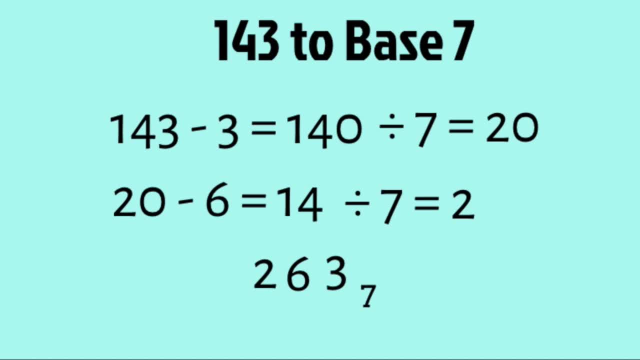 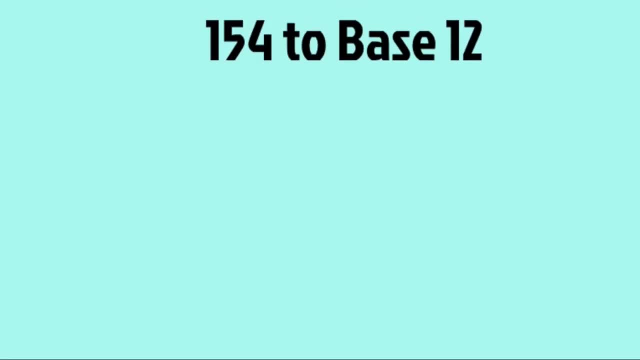 and since this value is less than 7, we just add it to the beginning of our number. Convert 154 to base 12.. Since 154 has a remainder of 10 when divided by 12, we subtract that off to get 144. 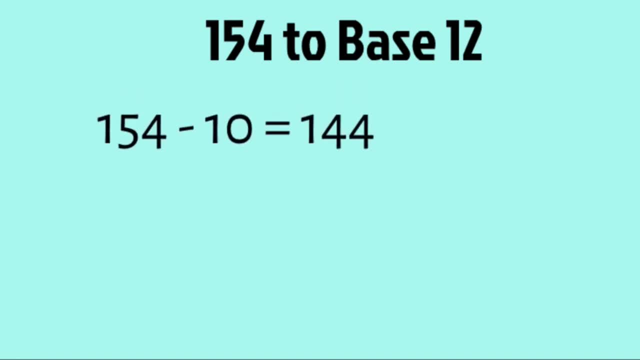 And, if you recall earlier, 10 is represented by A, so we add that to the end of our number, Then we divide by 12 to get a value of 12.. And since 12 has a remainder of 0 when divided by 12,, 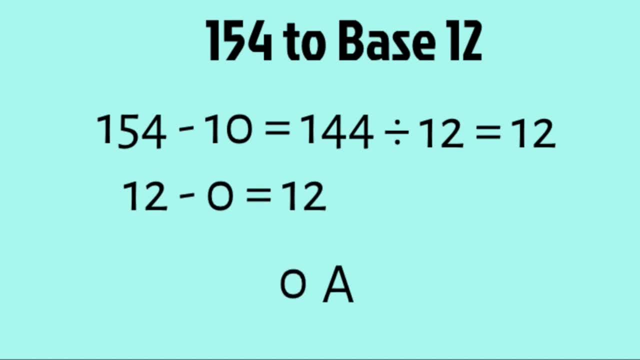 we subtract that off and get 12, and then we add a 0 to the beginning of our number. Then we divide by 12 to get 1, and since 1 is less than 12, we just add it to the beginning of our number. 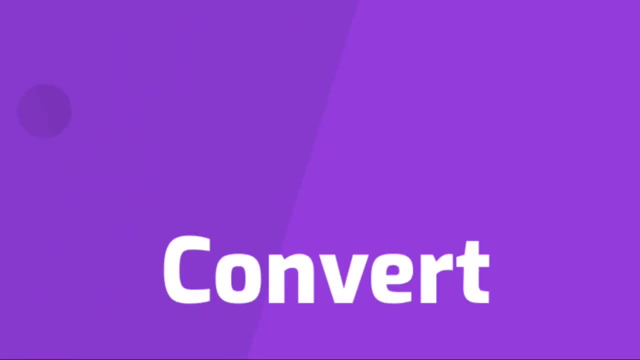 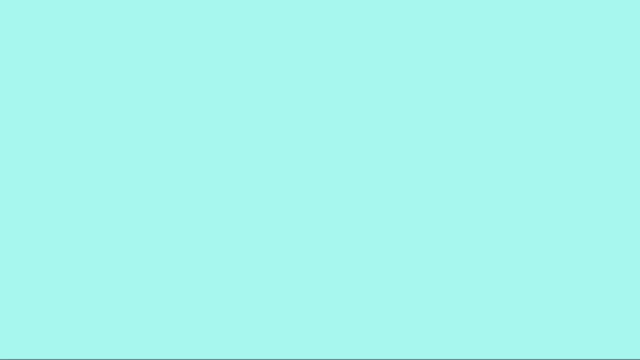 Finally, we will learn how to convert numbers between two bases that are both not 10.. Let's try an example: 162 base 7 to base 8.. First we convert 162 base 7 to base 10. We get a value of 93.. 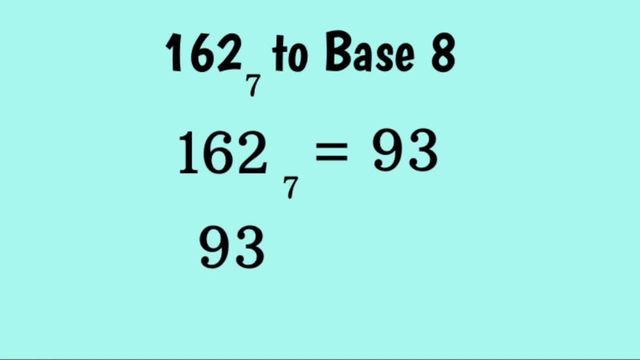 Then we convert 93 base 10 to base 8 to get a value of 135 base 8.. There are, however, some shortcuts to doing this. In order for this trick to work, one of the bases must be a power of the other. 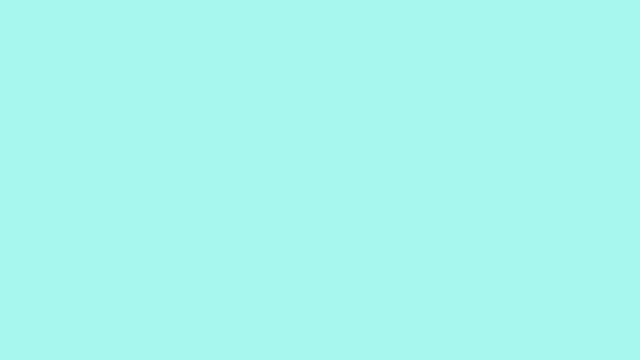 Let's try an example: Convert 110, 101, base 2 to base 8.. First we note that 2 to the 3 is equal to 8, so we must look for groups of three digits in our number. We can split our number up into two groups. 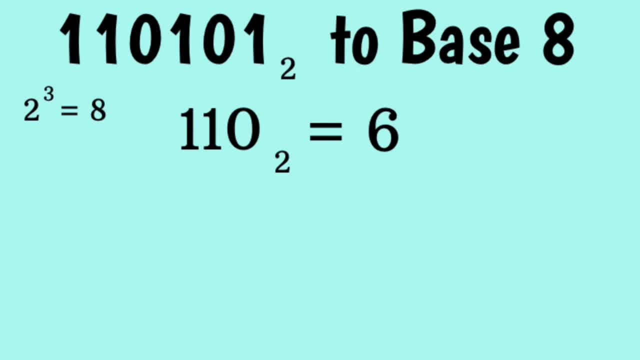 Our first group is 110,, so 110 base 2 is equal to 6.. Our second group is 101 base 2.. 101 base 2 is equal to 5.. So now what we must do is we must put our two digits together.